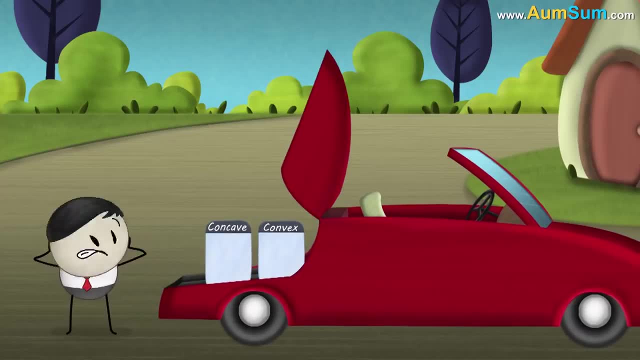 What an amazing car, But your rear view mirror is missing. No, Do not use a concave mirror. It will usually show you magnified images. Oh, Hahaha, Why don't you listen to me? Hm, See, I was correct. 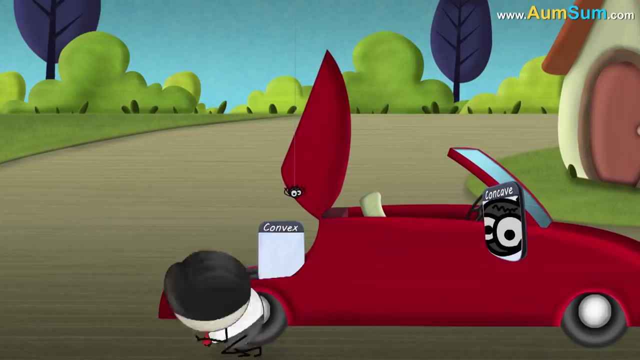 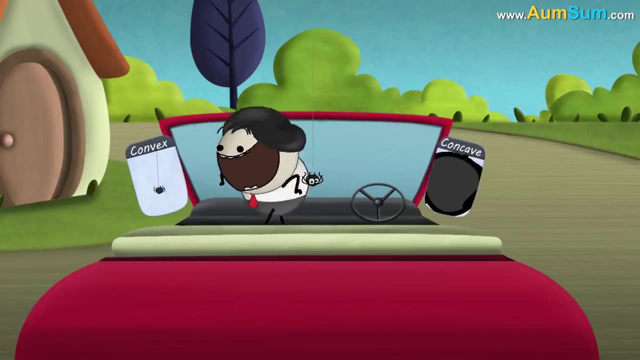 Now put the convex mirror and see the result. Look, the image is much smaller, right? Do you know what the difference between the two mirrors was? If we use a concave mirror for our car, We will not be able to see the vehicles behind us properly. 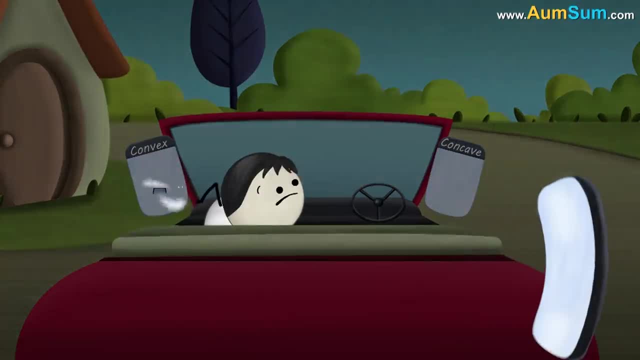 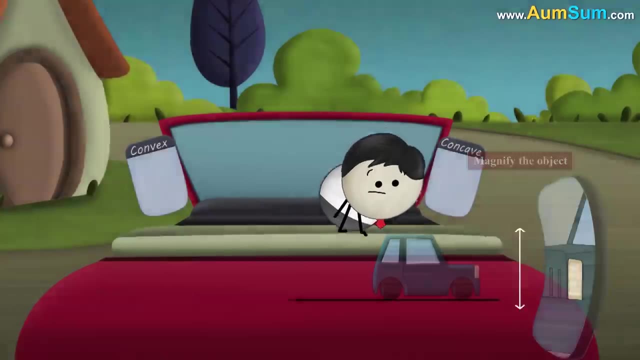 This is because the concave mirror will magnify the object And we will see a very enlarged image. Thus, we require a mirror which gives us a wider view of the vehicles behind us. In this case, a convex mirror proves to be the right choice. 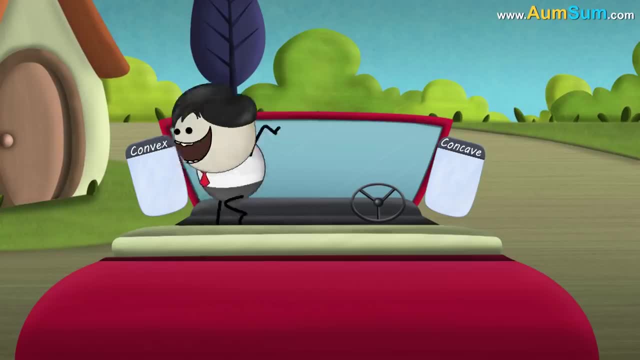 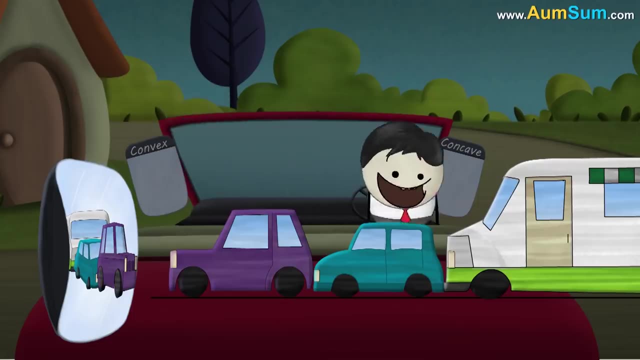 This is because a convex mirror forms a highly diminished image, Thus making the traffic look much smaller. As a result, we can see a large number of vehicles in a very small mirror. Now let us see how to make a convex mirror. 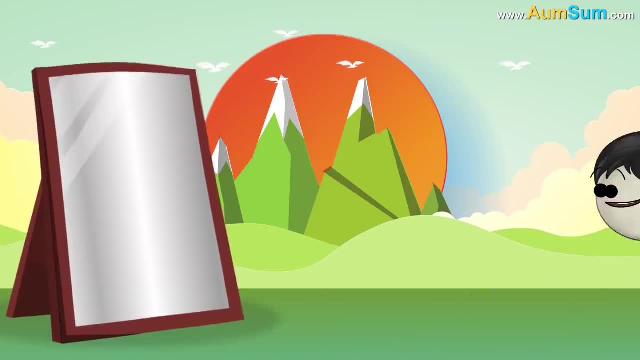 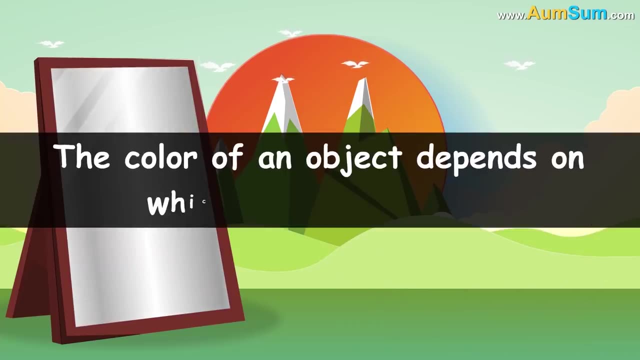 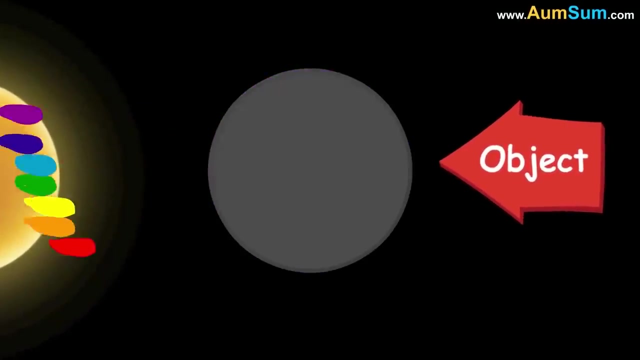 This is a very small mirror. What is the color of a mirror? Silver. No, The color of an object depends on which color it reflects. If an object reflects blue, it appears blue. If it reflects all colors, it appears white. 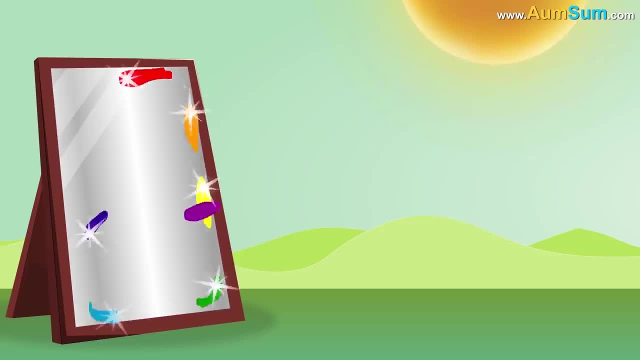 Now, a mirror reflects almost all colors, So that means its color should be white, Just like snow, right, But it is not. Snow scatters light in all directions, making it appear white, But the mirror doesn't reflect light the same way. 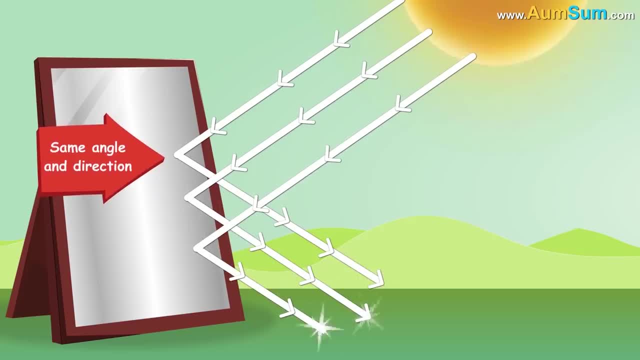 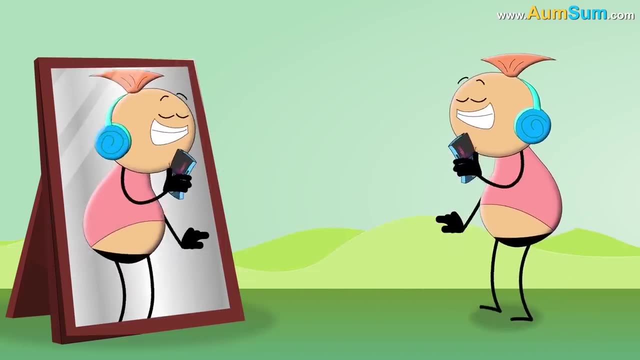 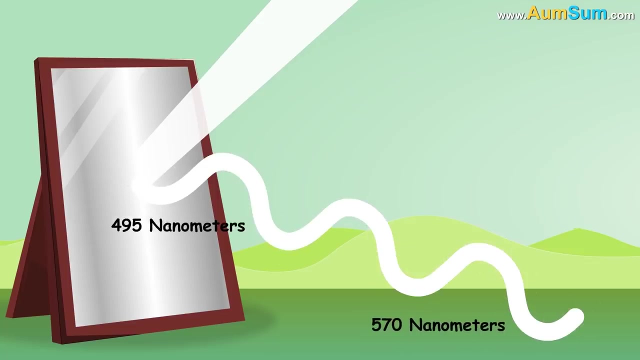 It reflects light at the same angle and direction from which it arrives. This is called specular reflection. Thus it creates an image of whatever is in front of it. Now, mirrors best reflect light at wavelengths between 495 and 570 nanometers. 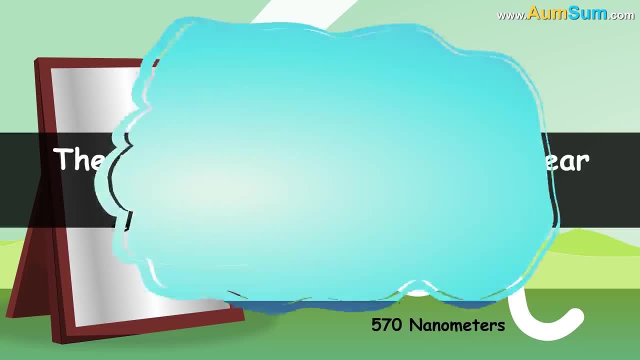 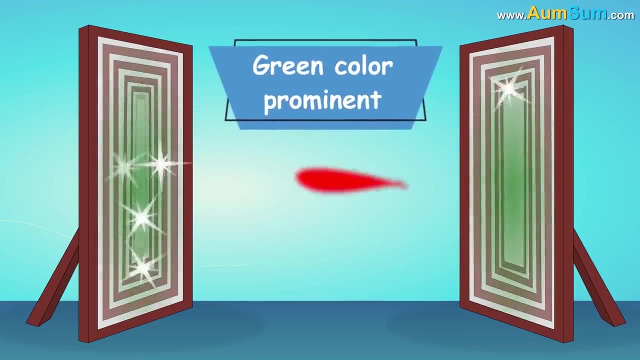 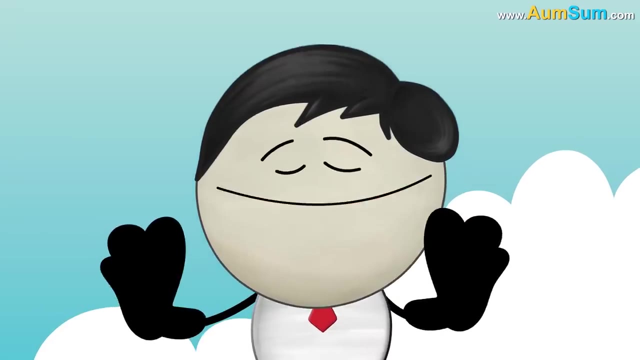 The wavelengths in this range appear green to us. We can observe this when two mirrors face each other. In this case, the same image is reflected back and forth, making green color prominent. What if mirrors disappeared? No problem, I am so handsome, I don't need a mirror. 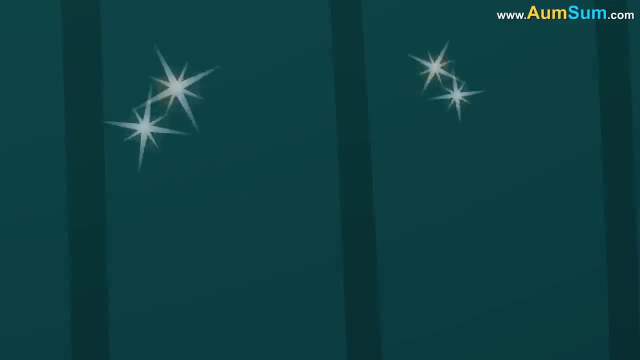 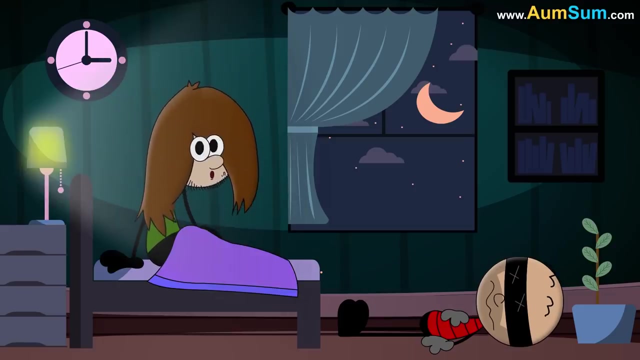 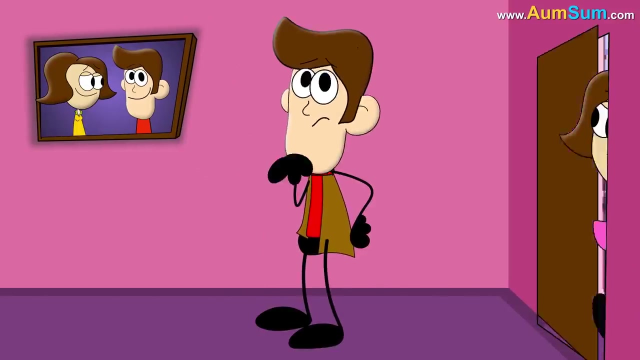 Oh AumSum. Firstly, if mirrors disappeared, People will rarely get haircuts, as they may fail to notice how long their hair have actually grown. Secondly, if mirrors disappeared, Ladies will not waste much time on makeup. Their husbands will be really happy. 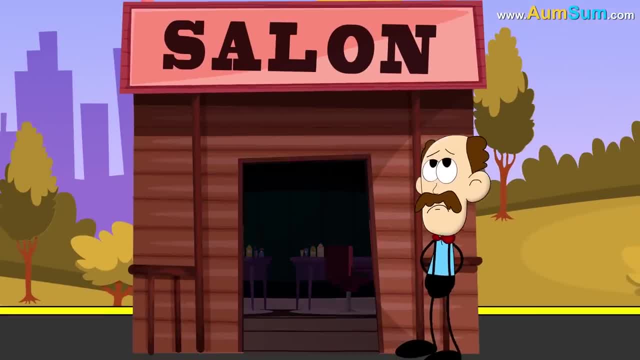 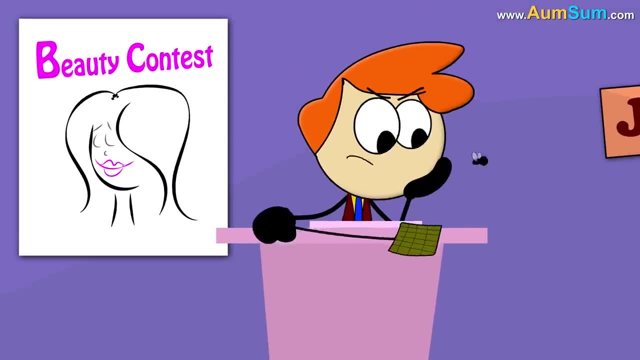 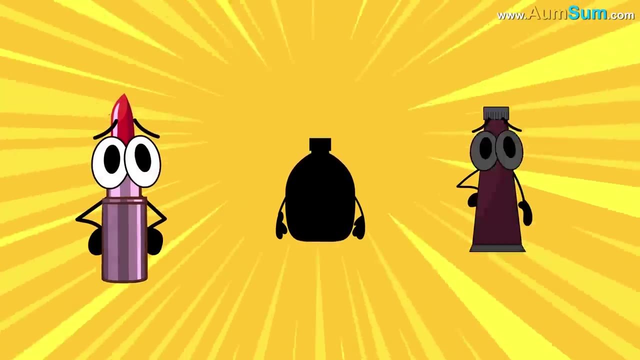 Thirdly, if mirrors disappeared, Salons might start closing down. Fourthly, if mirrors disappeared, Beauty contests may not be held anymore. Fifthly, if mirrors disappeared, Sales of cosmetic and beauty products like lipsticks, face creams, shampoos, etc. 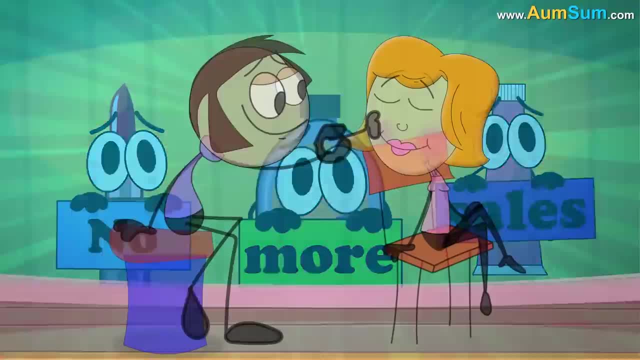 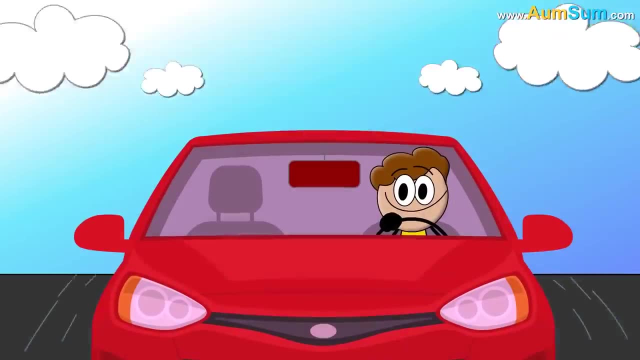 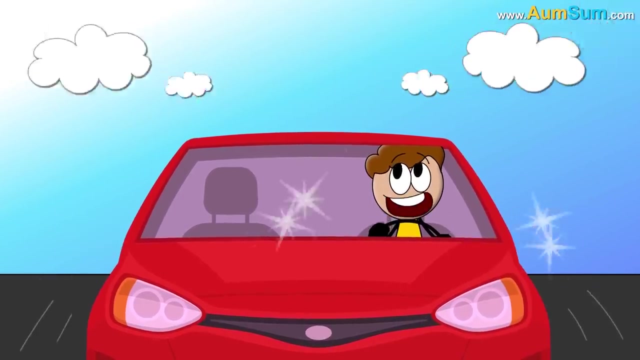 Will go down sharply. Sixthly, if mirrors disappeared, Makeup artists may have to look for a new profession. Lastly, rear view mirror, as well as side mirrors, are extremely important in cars. If mirrors disappeared, Driving a car may actually turn out to be dangerous. 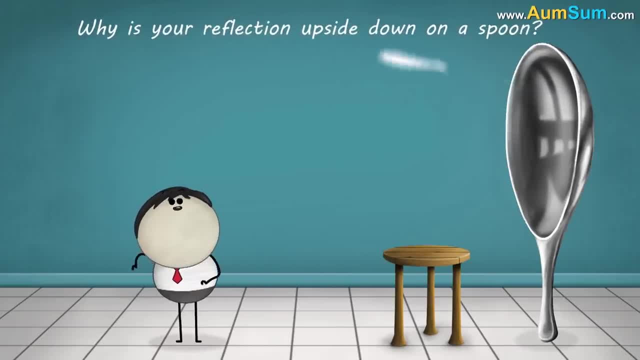 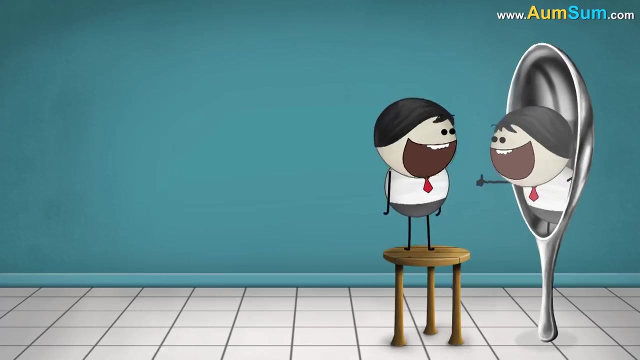 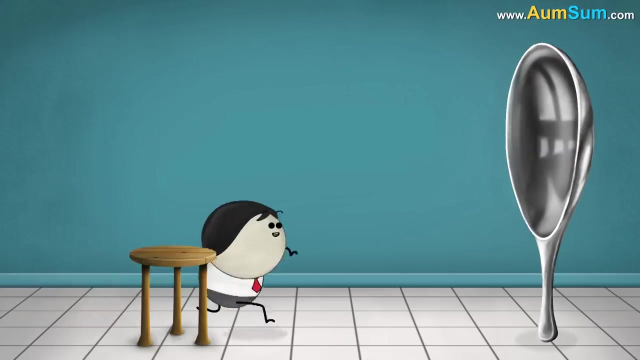 Concave mirror. Why is your reflection upside down on a spoon? Wow, Looks like you are getting ready to go for a party. Why don't you stand here and then look into the spoon? Don't worry, Your image appeared upside down because of the inward curve of the spoon. 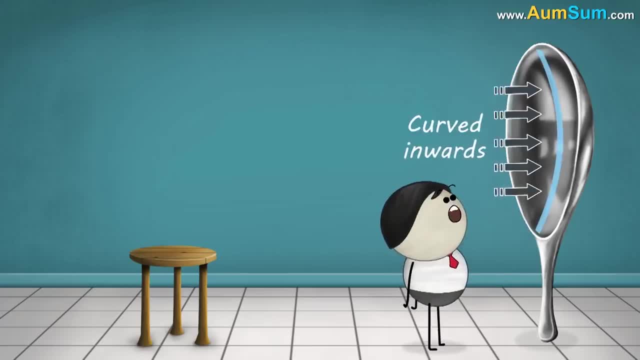 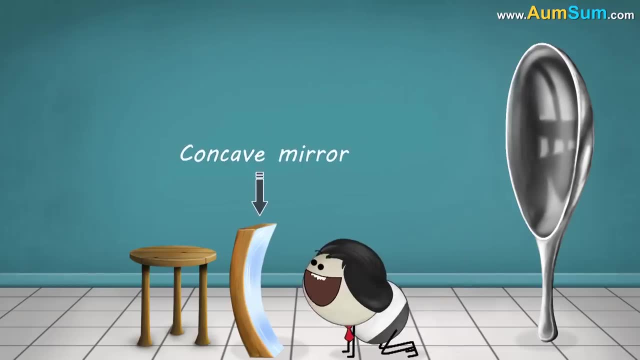 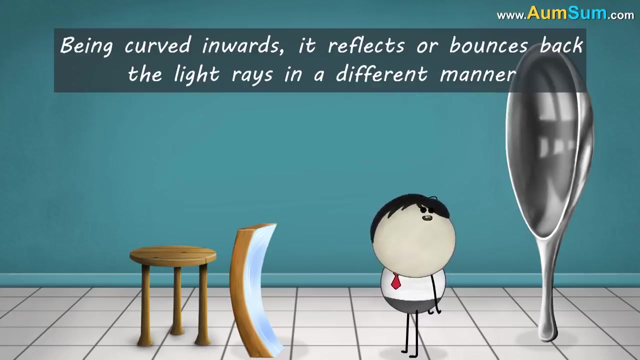 The surface of the spoon, which is curved inwards, acts like a concave mirror. You look confused. Let me explain. A concave mirror is a mirror whose reflecting surface is curved inwards. Being curved inwards, it reflects or bounces back the light rays in a different manner. 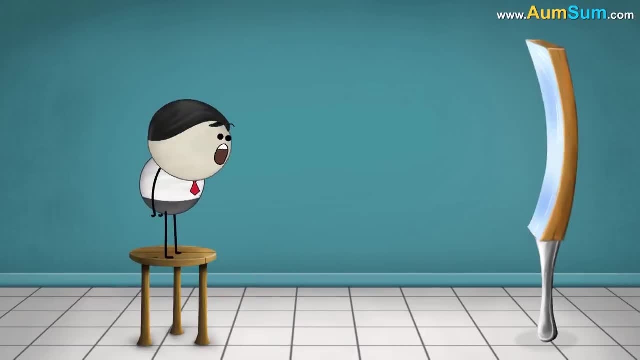 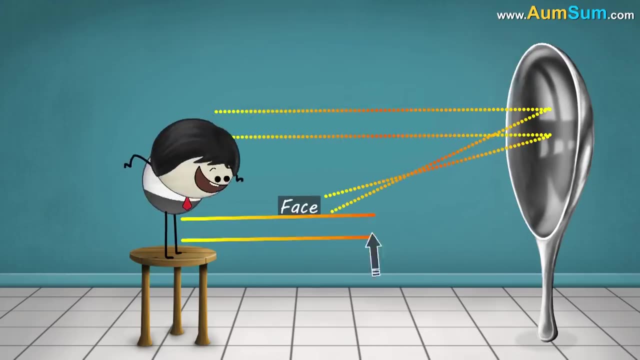 When you see yourself in a spoon which is like a concave mirror, The light rays from your face fall on the top of the spoon and get reflected downwards, While the light rays from your feet fall on the bottom of the spoon and get reflected upwards. 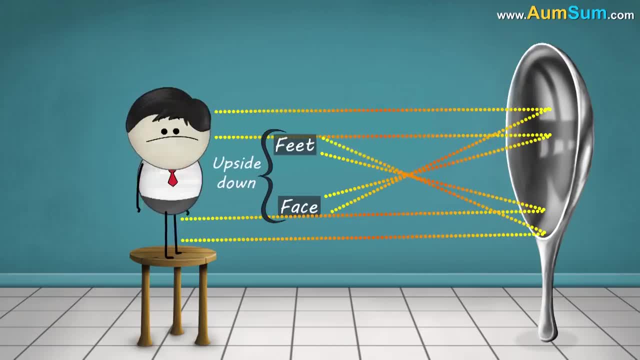 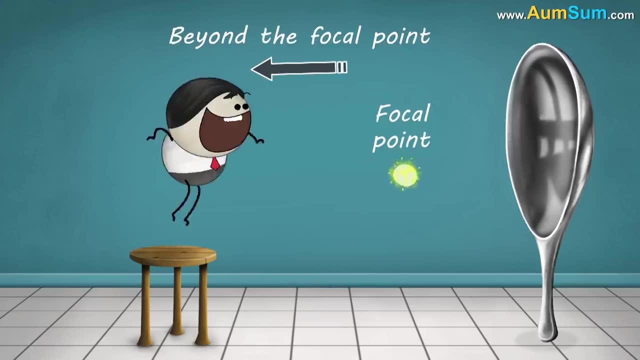 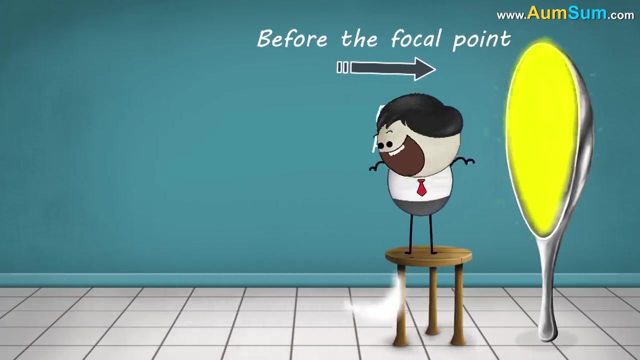 As a result, you see yourself upside down. Now, the point where all these light rays meet is called the focal point. When you stand beyond this point, only then will you be able to see an inverted image of yourself. However, if you stand before the focal point, the image will look upright. 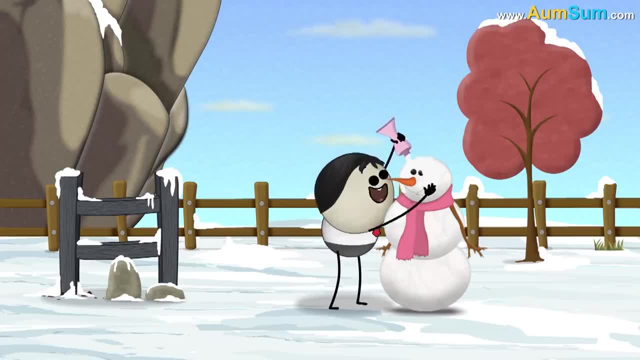 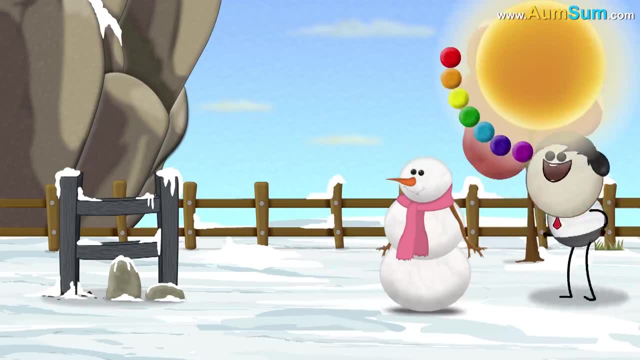 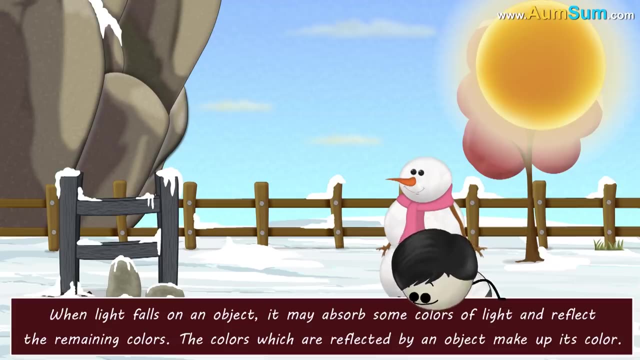 Why is snow white? Because it applies fairness cream. No Sunlight or white light is a combination of all visible colors of light. When light falls on an object, it may absorb some colors of light and reflect the remaining colors. The colors which are reflected by an object make up its color. 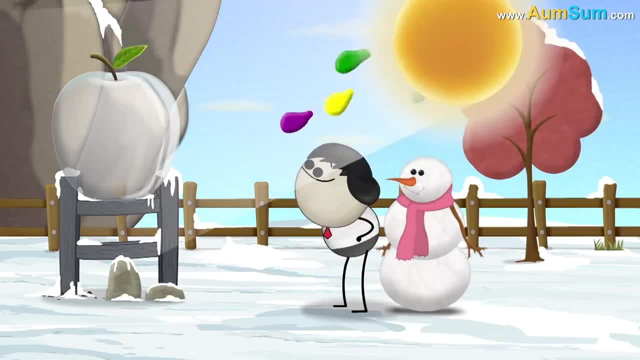 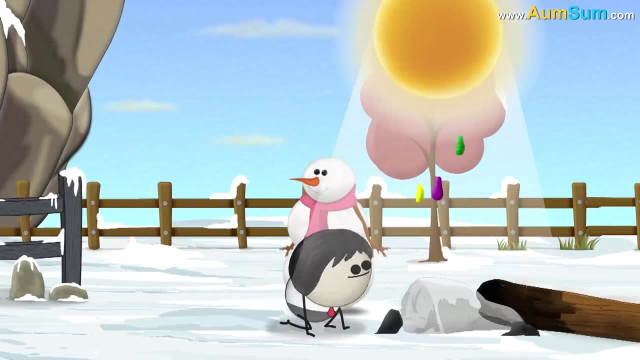 For example, when light falls on an apple, it absorbs all other colors except red. Apple reflects red color, making it appear red. When light falls on coal, it absorbs all colors and does not reflect any color. Hence Coal appears black to us. 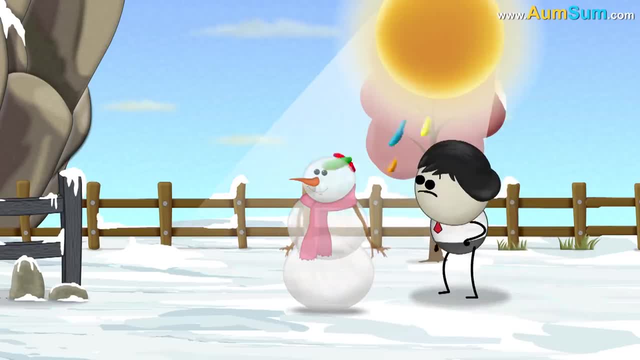 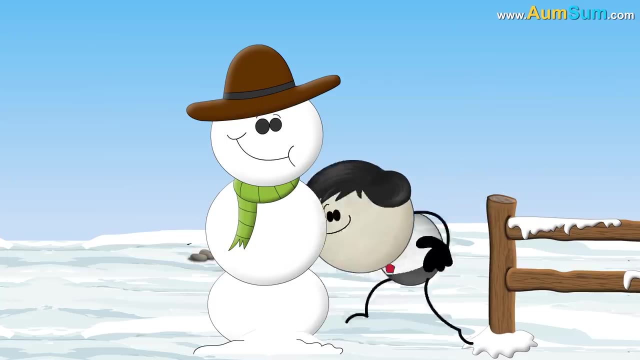 Really, I didn't know that Now. snow does not absorb any colors of light and reflects all of them equally, As the combination of all colors of light is white light, snow appears white to us. How do snowflakes form? My snowman makes them. 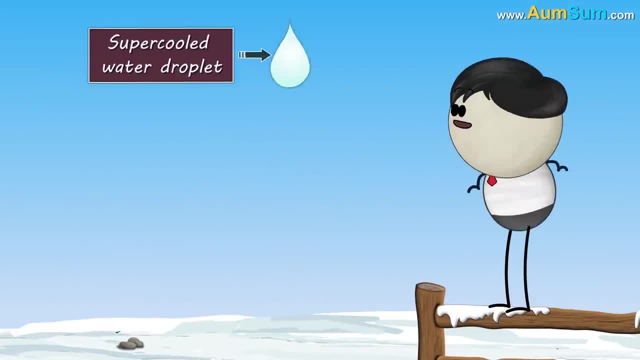 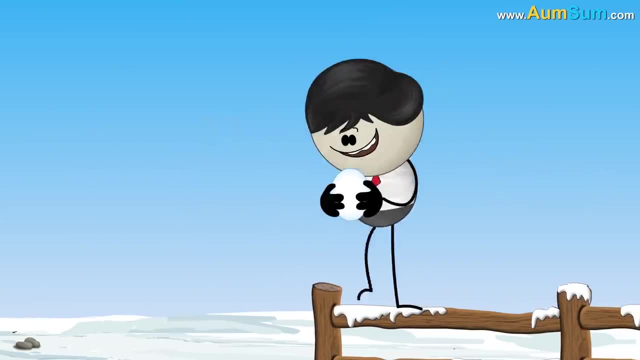 You wish. A snowflake begins to form when a supercooled water droplet in the sky. It freezes onto a dust particle or pollen, forming a tiny ice crystal. However, when water freezes, its molecules arrange themselves in a hexagonal pattern. 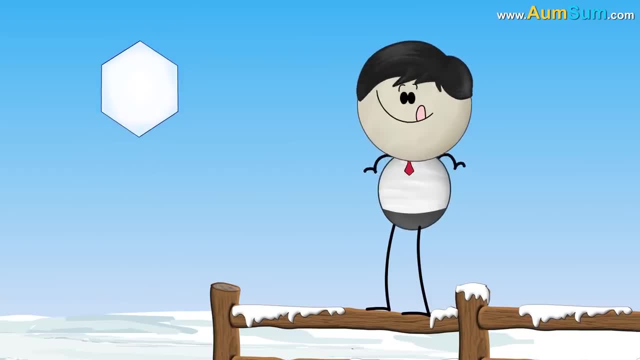 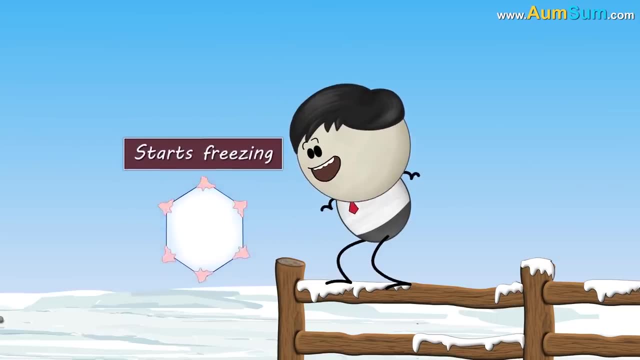 Thus giving the crystal a hexagonal shape. Now, as the ice crystal keeps falling, it comes in contact with more water. As a result, the water starts freezing on the six corners of the ice crystal, Causing branches to grow on the corners and thus giving us a beautiful snowflake. 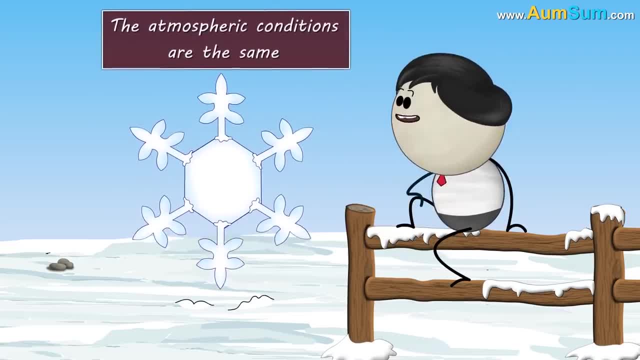 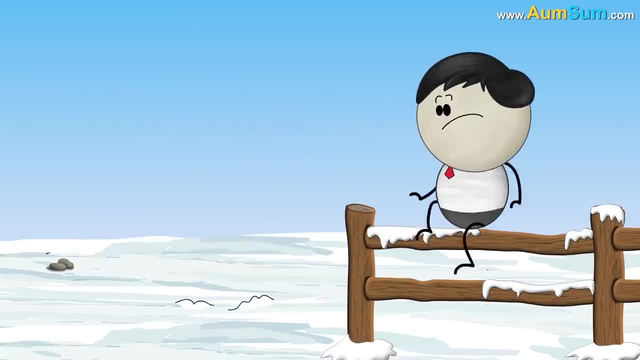 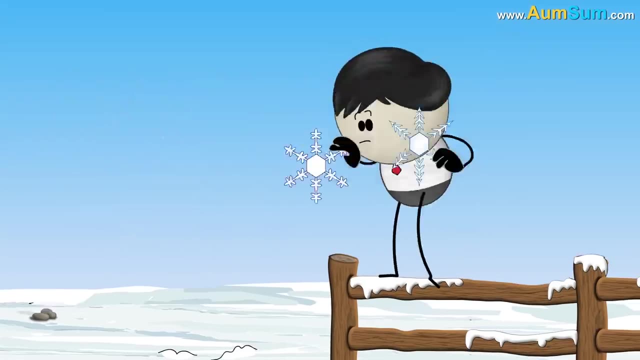 Also, as the atmospheric conditions are the same on all sides of the snowflake, The branches grow identically, thus making the snowflake symmetrical. But since every snowflake follows a different pattern to the ground, It encounters different atmospheric conditions. Hence it is said that no two snowflakes are the same. 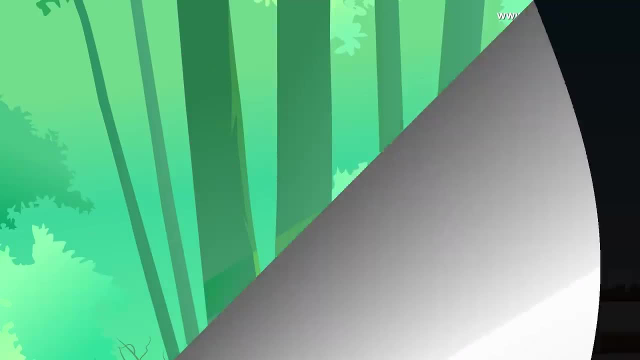 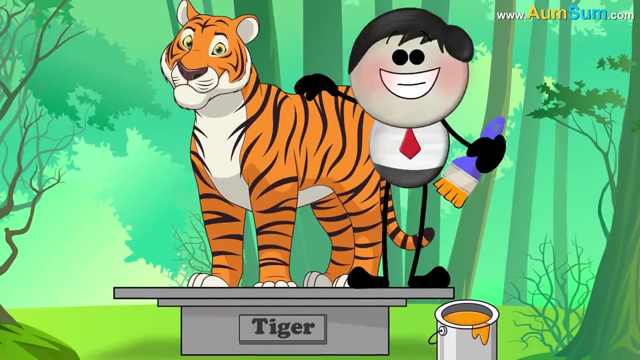 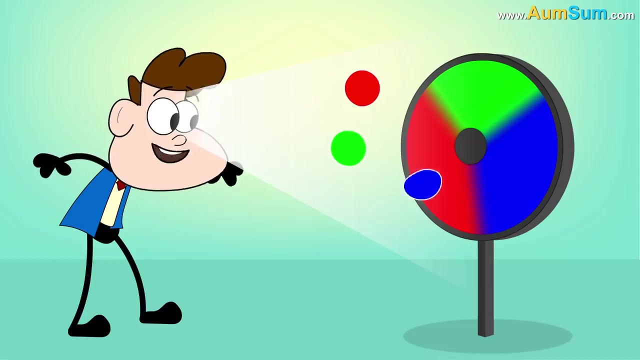 They all tend to be unique. Why are tigers orange in color? Simple, I painted them orange, Oh AumSum. Humans are trichromats, As in their eyes, can process red, green as well as blue colors. Hence to humans, the tiger appears orange in color.